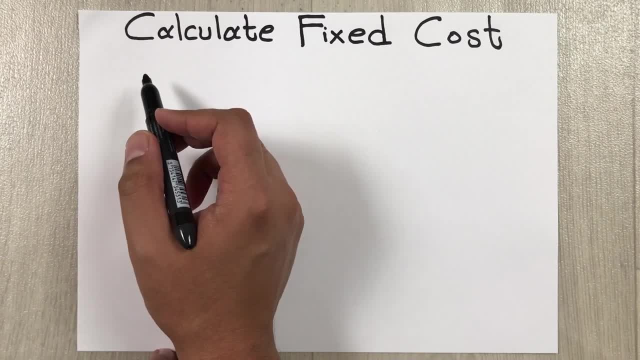 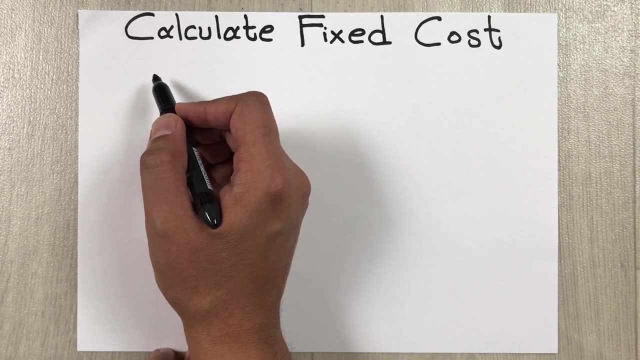 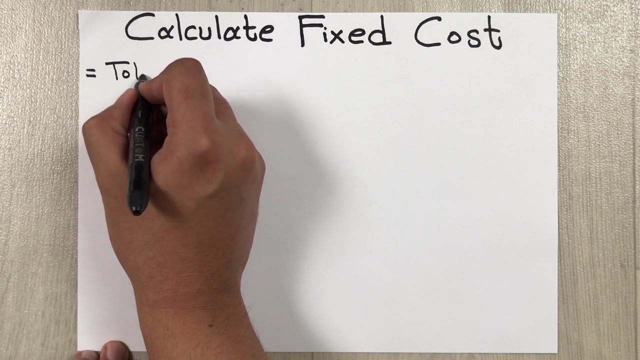 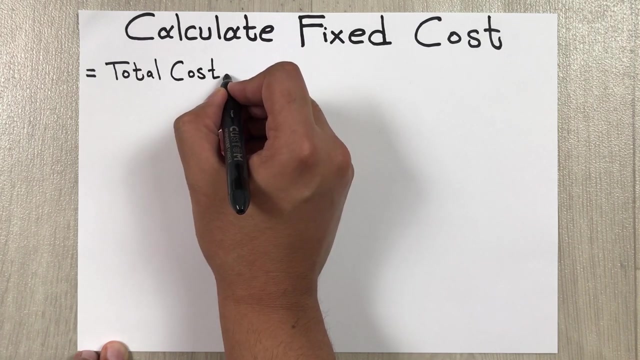 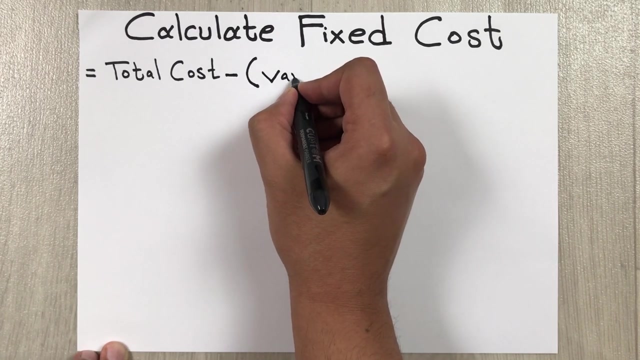 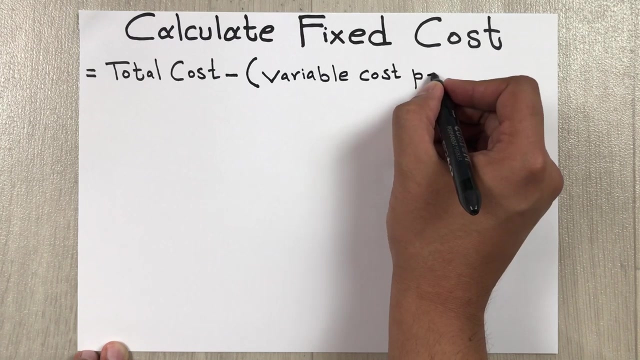 hello, guys, i hope you are doing really, really well. in today's video i'm going to show you how to calculate fixed cost. so, guys, the formula to find out the fixed cost is equal to total cost minus. then we put the bracket: variable cost per unit. variable cost per unit. 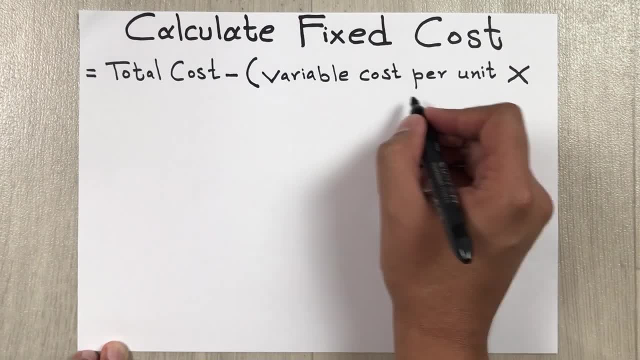 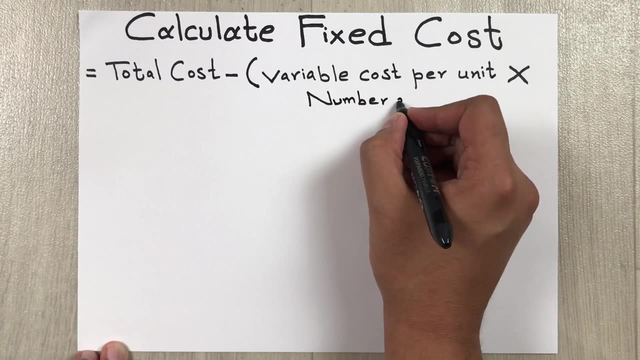 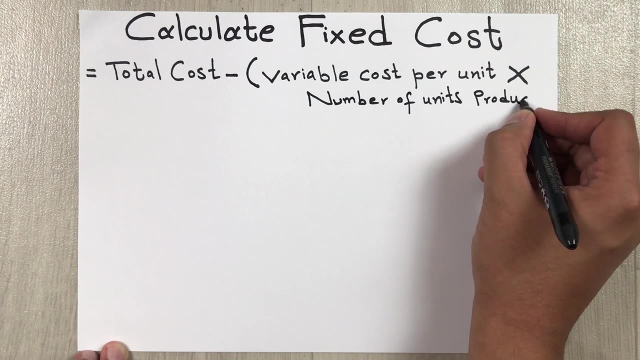 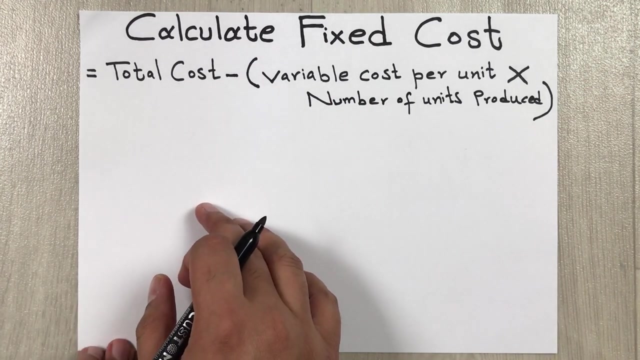 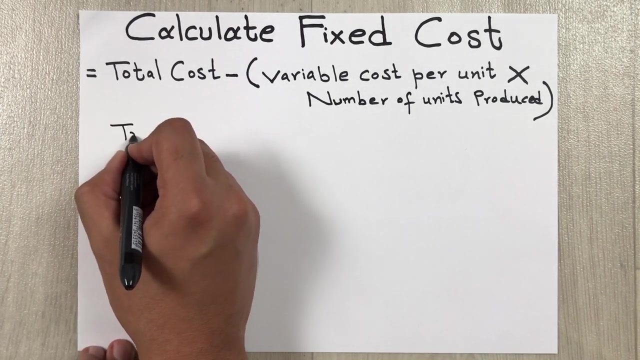 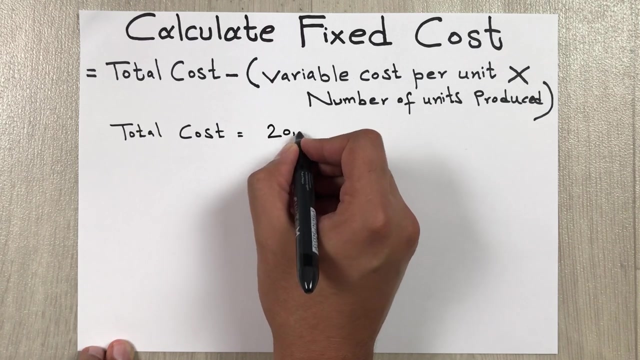 multiply by number of units. okay, multiply by number of units produced, and then we close the bracket. so, guys, this is the formula. so, guys, let's say the total cost of production is twenty thousand dollars. okay, so total cost is equal to twenty thousand dollars and the variable cost per unit is five. 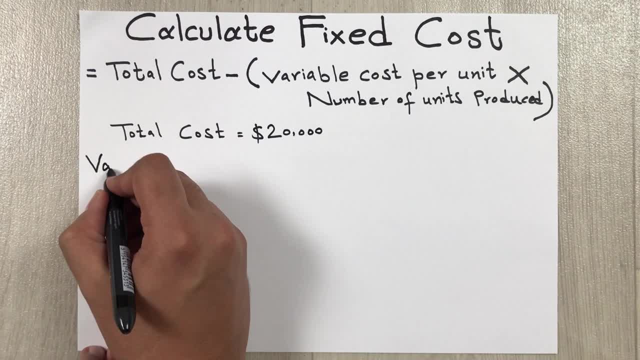 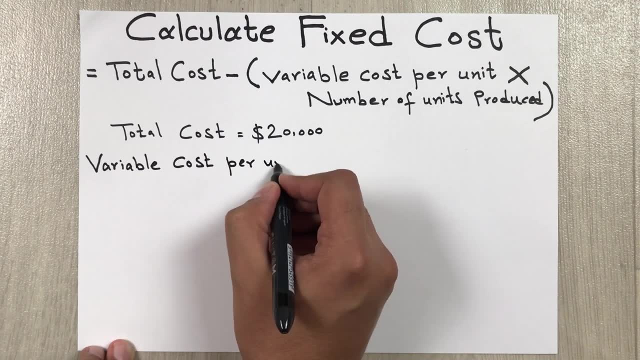 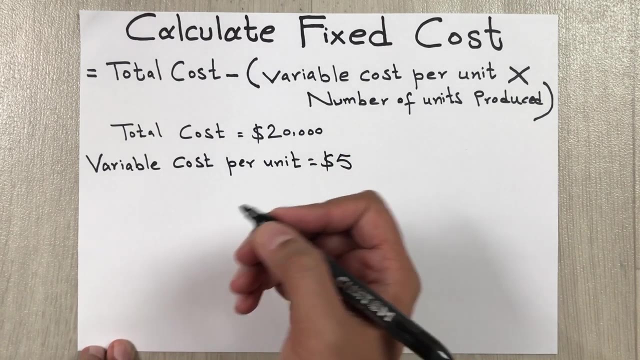 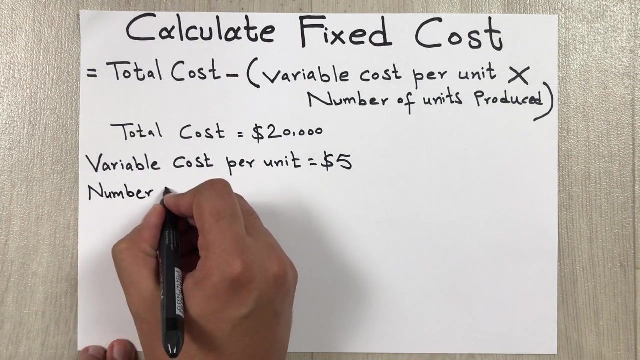 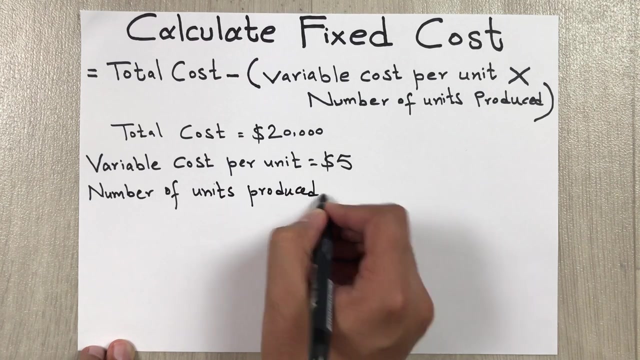 dollar, variable cost per unit is equal to five dollars. ok, and the number of units produced like this is the total cost of the unit. let's say 3,000, 3,000, number of units produced, so that we already get all values. we just simply put into the formula. then we will get our answer. so 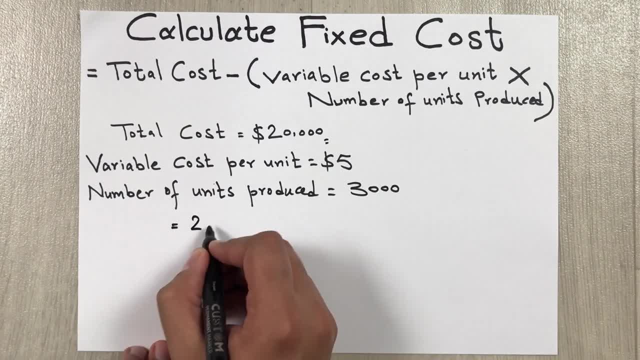 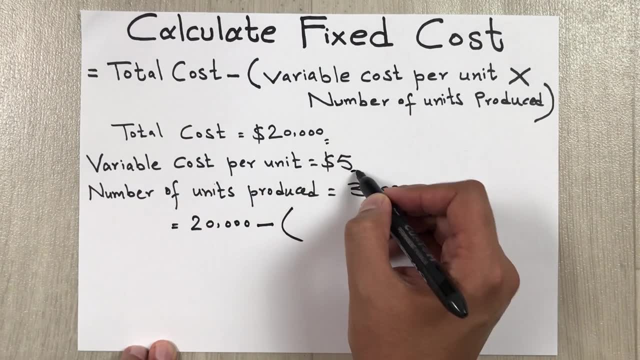 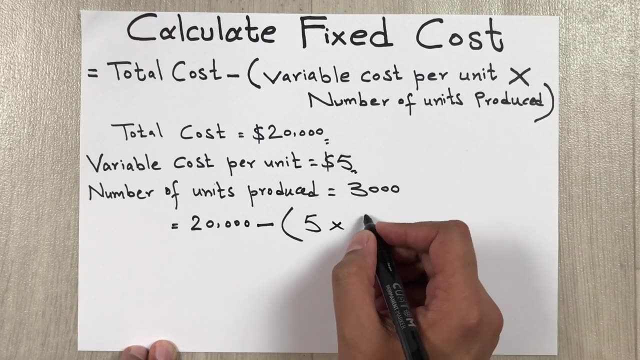 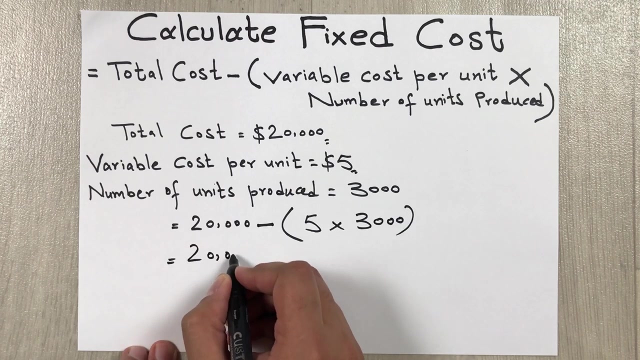 total cost is 20,000, so we put here 20,000. okay, then minus variable cost per unit, over here we have five dollars. so five and multiply with number of units produced, so multiply with 3,000. okay, then we do the simplification, so 20,000.